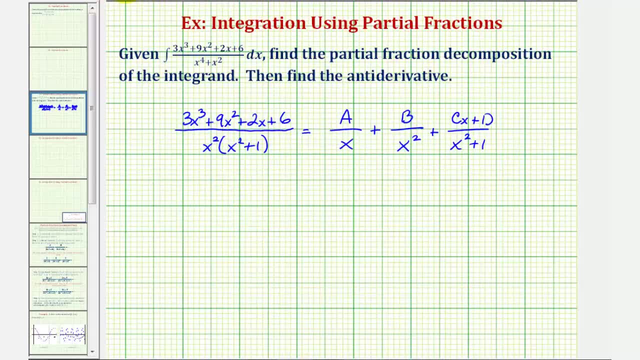 to determine the partial fraction decomposition. So the next step is to clear the fractions from our equation, which will give us what's called the basic equation, and we'll do this by multiplying both sides of the equation by the LCD, which would be x squared times the quantity x squared plus one. 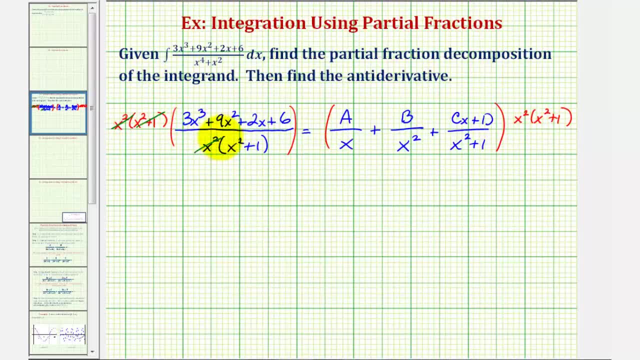 So on the left side, notice how these factors divide out, leaving us with three x to the third plus nine x squared, plus two x plus six. Now we need to be careful here. on the right, Notice how, for this first product, this product, here, one factor of x would simplify out. 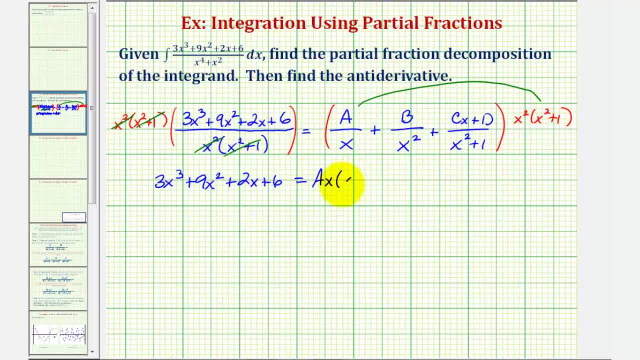 leaving us with ax times the quantity x squared plus one. Now for the second product. notice how the x squareds divide out, leaving us with b times the quantity x squared plus one. And then for the third and final product. notice how the factor of x squared plus one simplifies out. 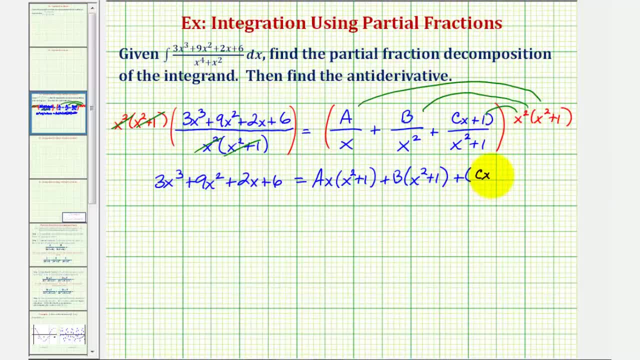 leaving us with plus cx, plus d times x squared. Now, to help us determine the values of a, b, c and d, we'll use the process of equating the coefficients. So for the next step, we'll multiply out the right side of this equation. 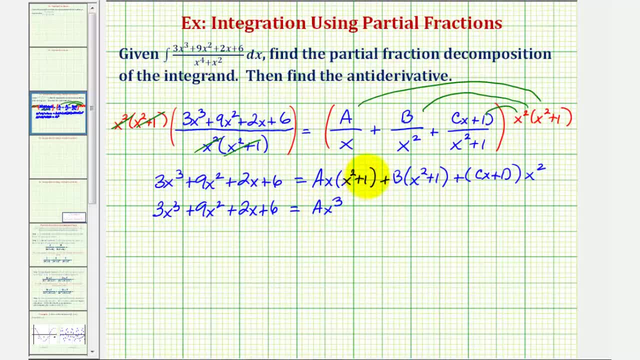 So we'd have ax to the third plus ax. Here we'll have plus bx squared, And here we'll have plus cx to the third plus dx squared, And here we'll have plus cx to the third plus dx squared, And now we'll group the x cubed terms together. 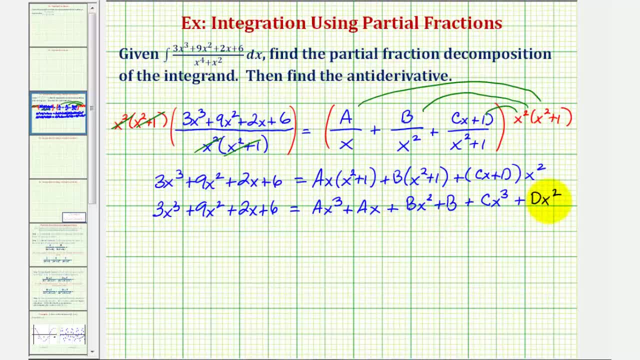 x squared terms together, x terms and constants. So notice how there are two x cubed terms here and here. Let's go ahead and factor out the x cubed. So if we factor out the x cubed and we put the x cubed to the right, 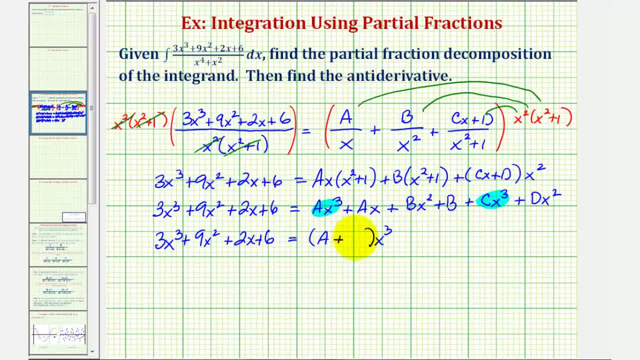 notice how we'd have a plus c as the coefficient. Next are our two x squared terms. We have plus bx squared plus dx squared, So if we factor out the x squared, we'd have the quantity b plus d times x squared. Notice how there's only one x term and one constant term. 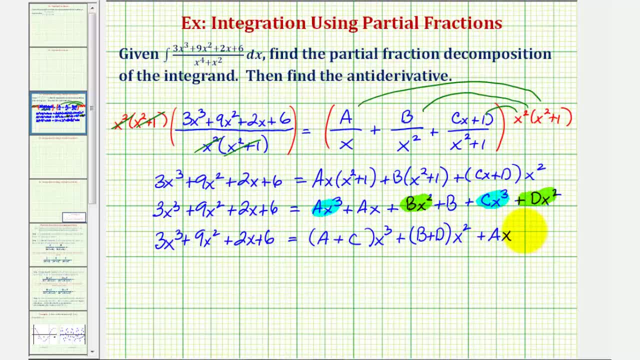 So we have plus ax squared plus dx squared, Bx plus b. And now, because the coefficients on the left must be equal to the coefficients on the right of the like terms, notice how we have: a plus c must equal three, B plus d must equal nine. 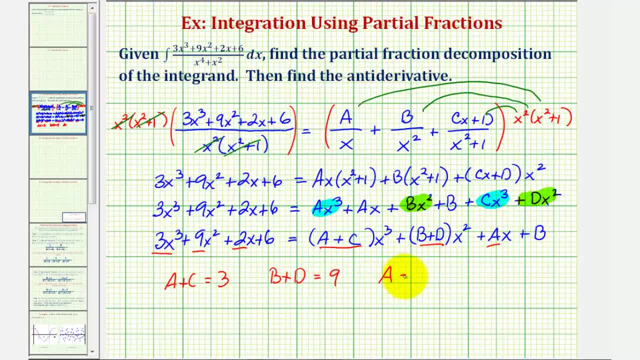 A must equal two And finally, b must equal six. Well, notice, if a equals two and a plus c equals three, we know c equals one. And if b plus d equals nine and we know b equals six, we know d must equal three. 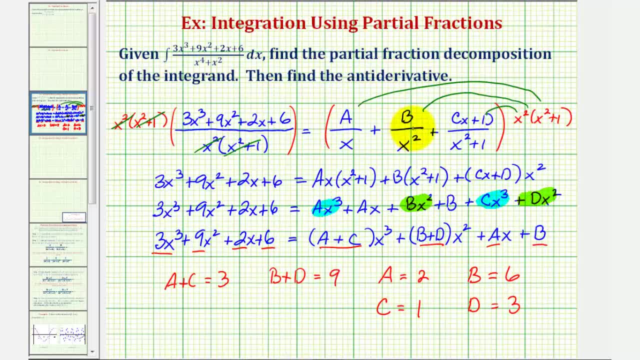 Now that we know the values of a, b, c and d, we'll perform these substitutions here, on the right side of this equation, which will give us our partial fraction decomposition. Let's go and do this on the next slide: The partial fraction decomposition of the integrand. 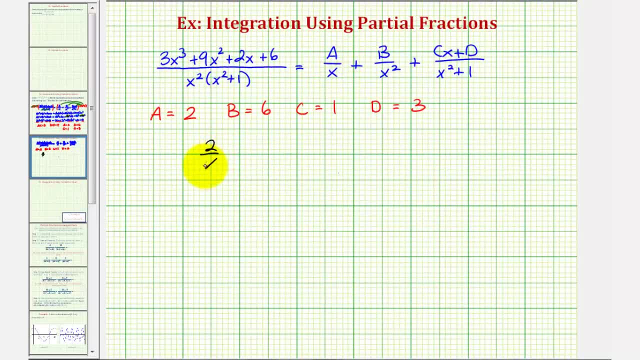 would be a divided by x, or two divided by x plus b divided by x squared, or six divided by x squared plus cx plus d divided by the quantity x squared plus one. And since c is one and d is three, we'd have the quantity x plus three. 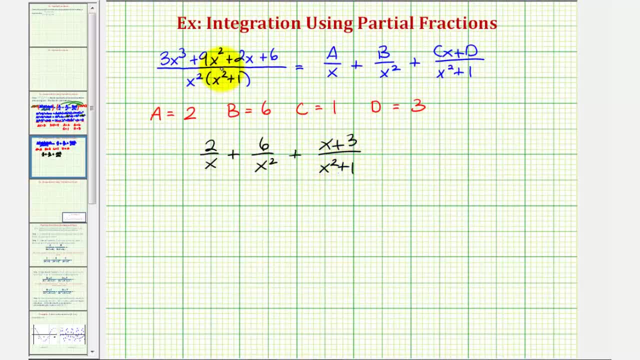 divided by the quantity x squared plus one, which means we can now find the antiderivative in this form rather than this form. So now our new problem is: we want to find the integral of two divided by x plus six divided by x squared plus the quantity x plus three. 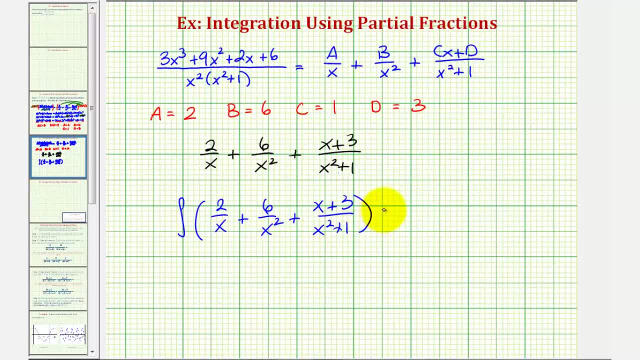 divided by the quantity x squared plus one with respect to x. Before we do this, though, notice how we'll have to change the form of this term by moving this up into the numerator and writing this as six x to the power of negative two. 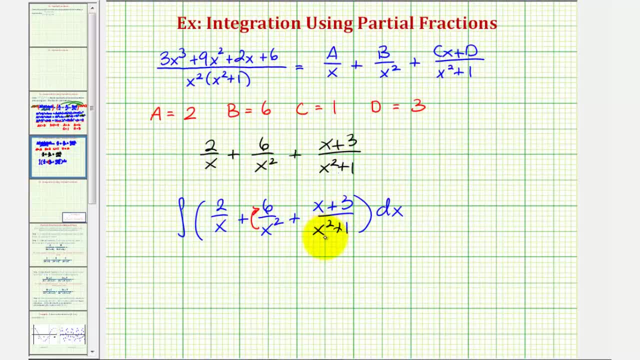 And notice how, for this third term, your substitution is not going to work in this form. We'll have to write this as two separate fractions, So write this as the integral of two divided by x plus. we'll write this as six times x. to the power. 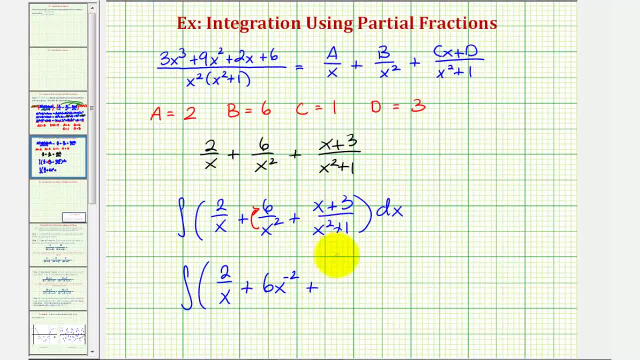 of negative two plus here we'll write x divided by the quantity x squared plus one plus three divided by the quantity x squared plus one. Now we'll break this up into four separate integrals to find the antiderivative, To save a little bit of time. 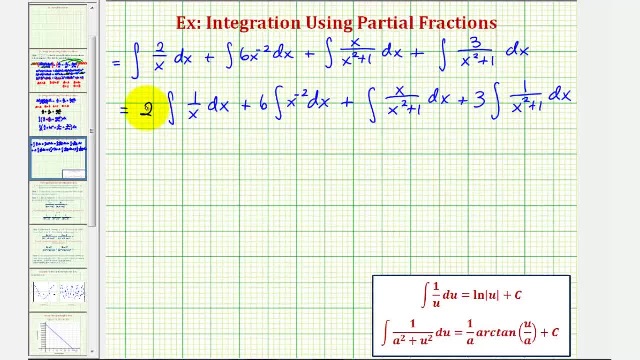 I wrote this as four separate integrals and then notice how I factored out the two here, the six here and the three here. Now we'll find our antiderivatives. So we'd have two times the integral of one over x. 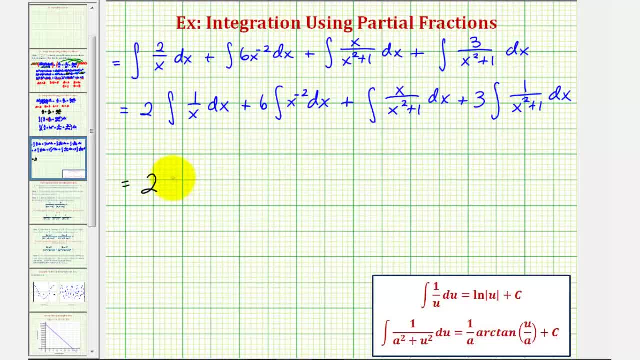 is equal to natural log absolute value of x. So we have two natural log absolute value of x plus here we'd have six times. we'll add one to the exponent, that would be x to the power of negative one divide by the new exponent that's going to be negative one. 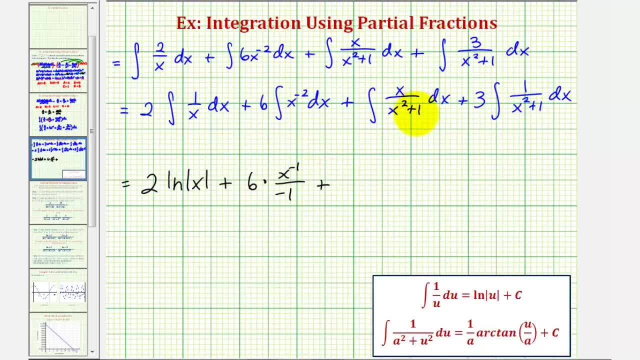 plus, here we'll perform u substitution where we'll let u equal the denominator. So notice: if u is equal to the denominator of x, squared plus one differential, u equals two x dx. notice how we only have x dx. So if we divide both sides by two, 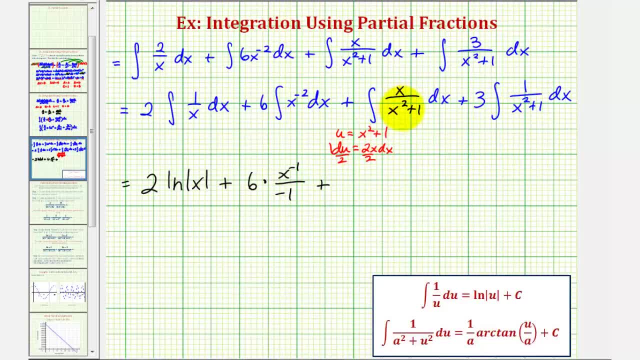 write this in terms of u, we'll have an extra factor of one half. This would be equal to one half times the integral of one over u du. So the antiderivative would be one half natural log absolute value of x squared plus one. 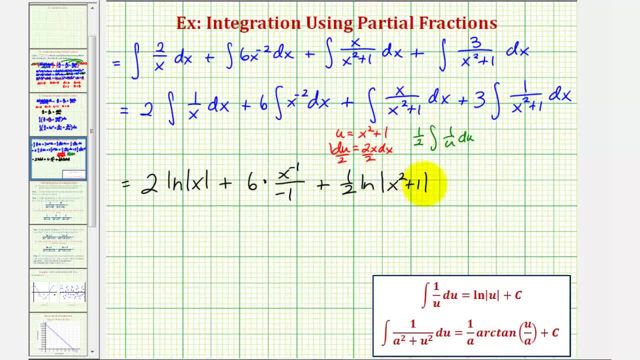 Notice how here, x squared plus one is always positive, so the absolute value is not necessary here. Now for the last integral. we'll use the integration formula given here below. Notice how our antiderivative will involve arc tangent. where a squared equals one, u squared equals x squared. 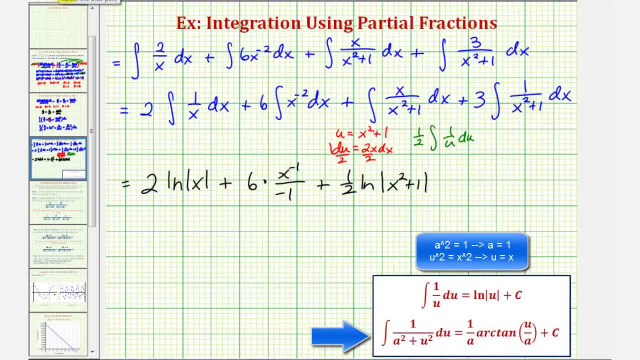 so u is x and a is one and therefore the antiderivative would be plus three times one over a, which is just one. and then we have arc tangent of u divided by a, which would be x divided by one, which is just x. 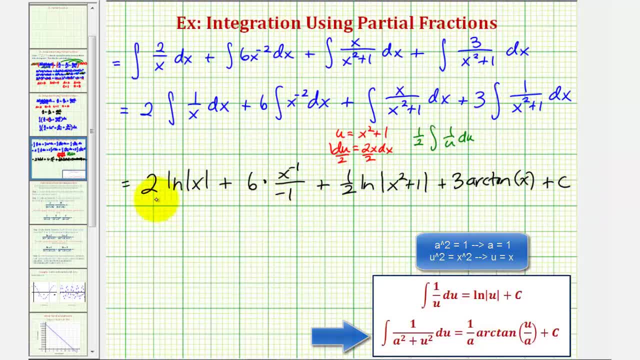 and of course plus c. Let's simplify this one more time. So we have two natural log absolute value of x. Here we'd have minus six over x, and then we have plus one half natural log. Again, the absolute value here is not needed.